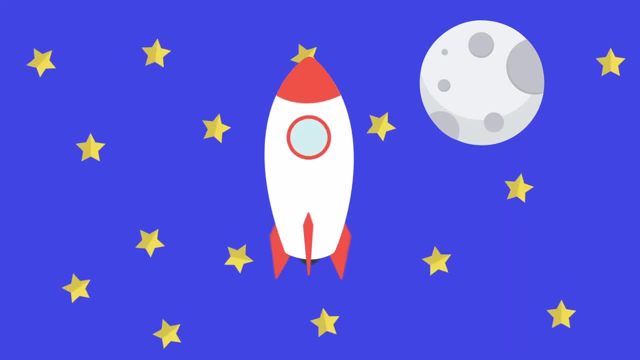 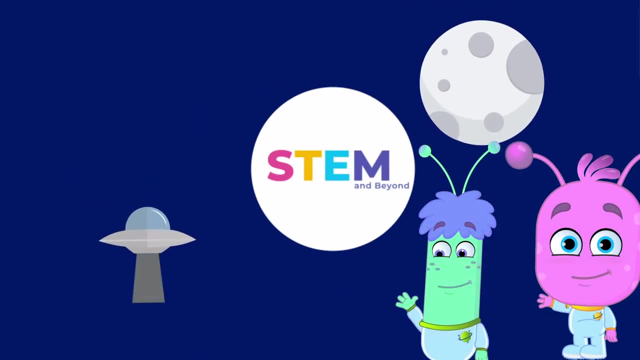 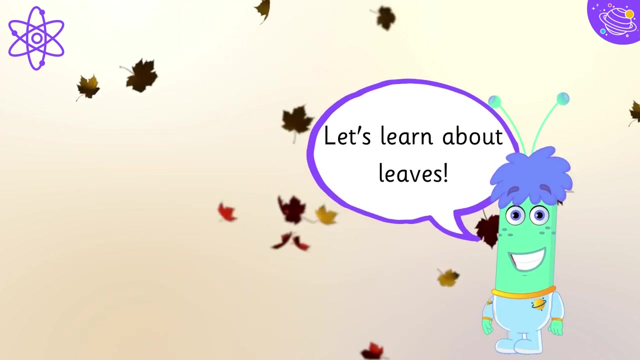 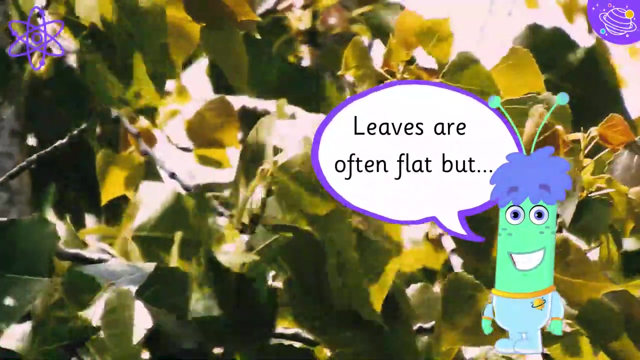 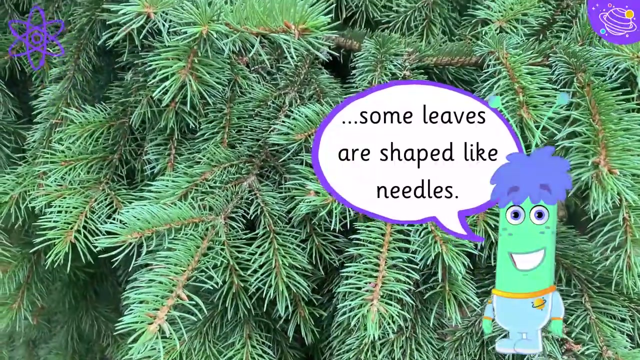 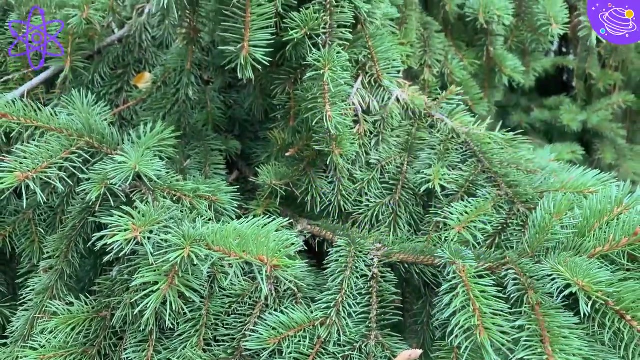 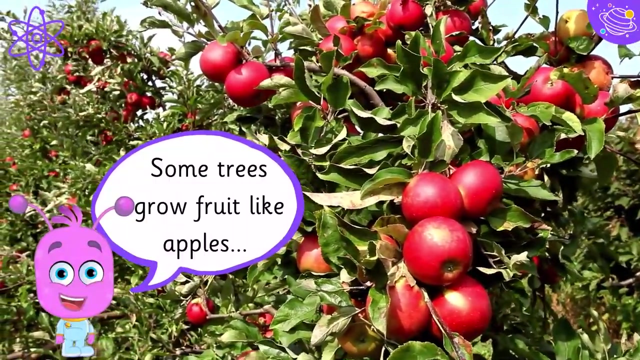 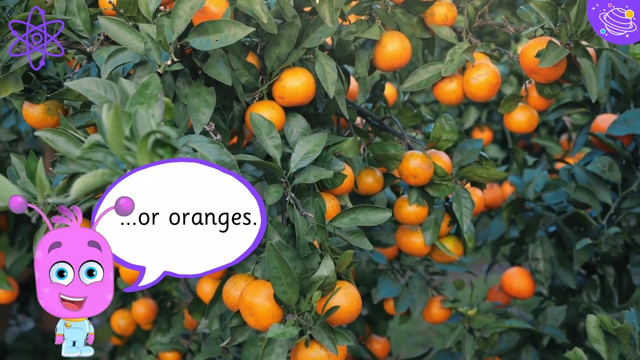 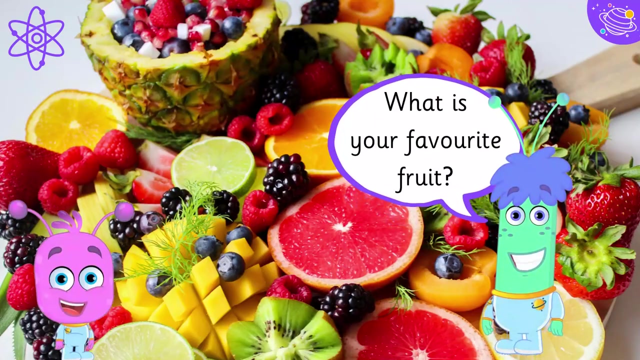 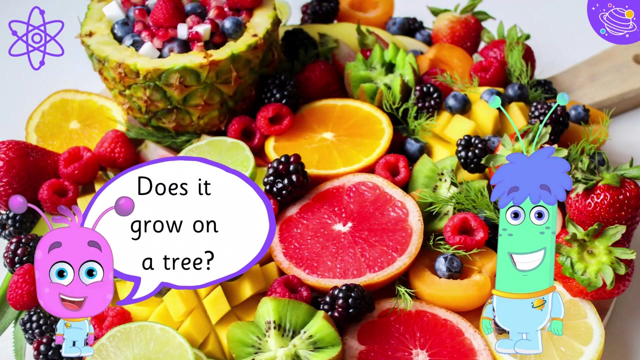 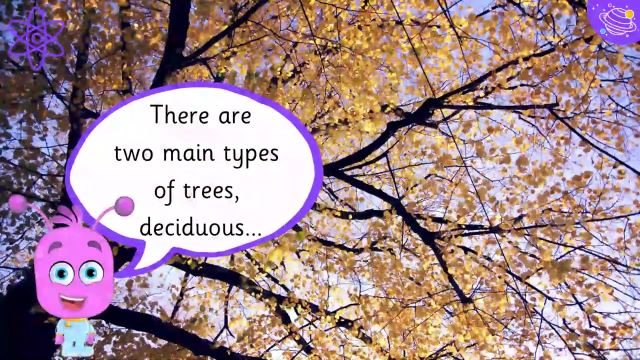 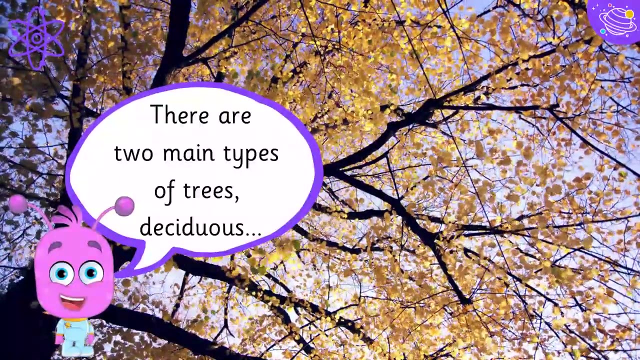 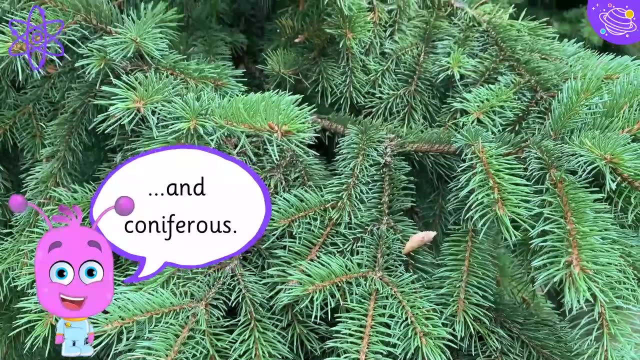 Let's learn about leaves. Leaves are often flat, but some leaves are shaped like needles. Some trees grow fruit, like apples or oranges. What is your favourite fruit Does it grow on a tree? There are two main types of trees: deciduous and coniferous. 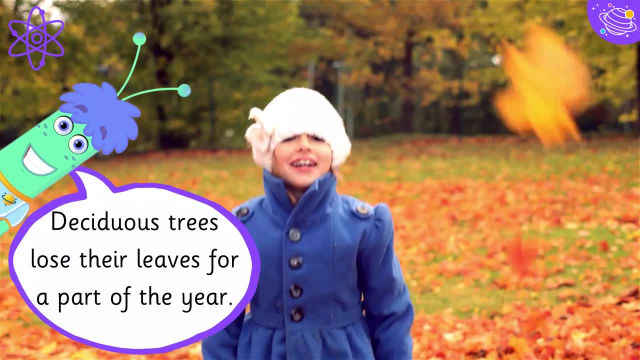 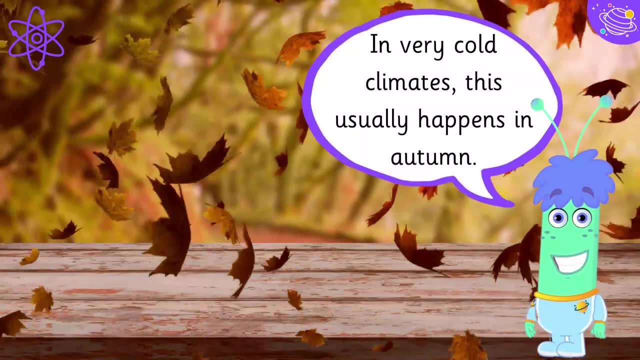 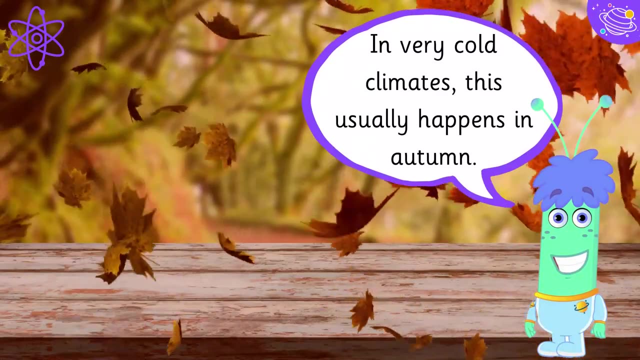 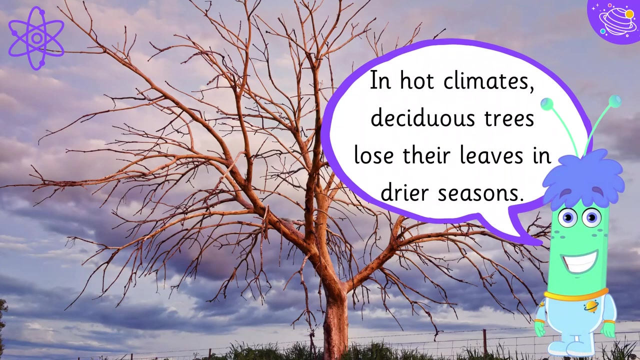 Deciduous trees lose their leaves for a part of the year. Deciduous trees lose their leaves for a part of the year In very cold climates. this usually happens in autumn In hot climates. deciduous trees lose their leaves in drier seasons. 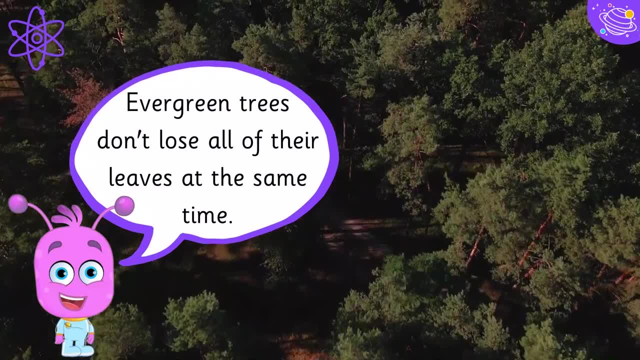 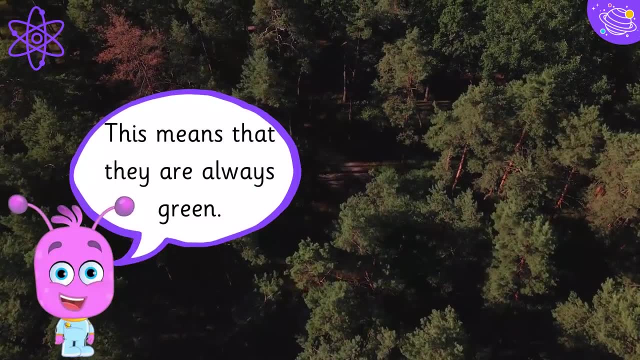 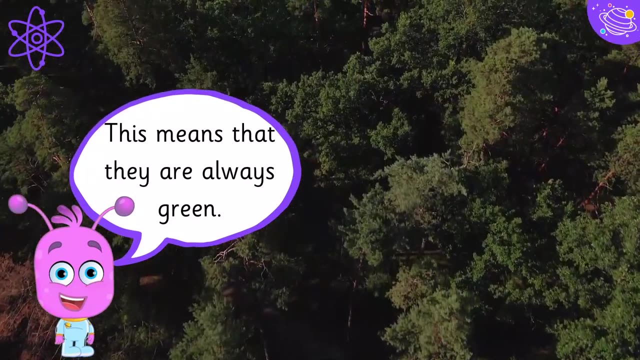 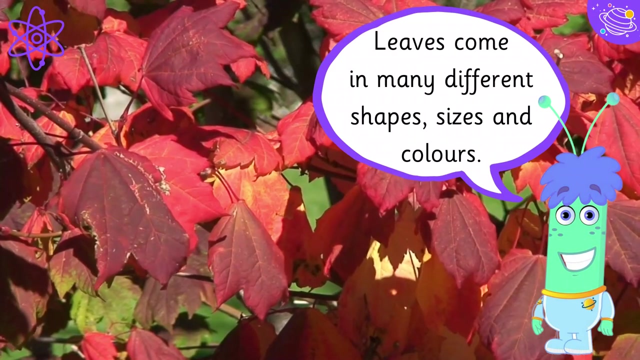 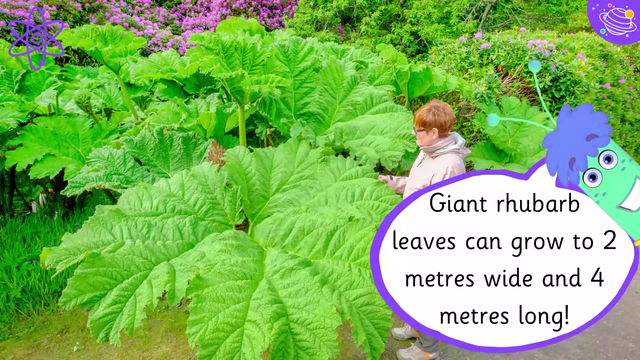 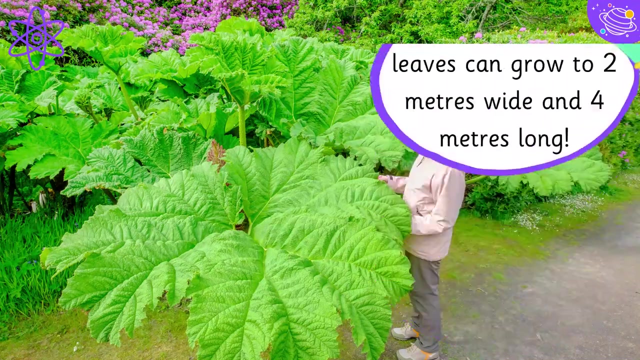 Evergreen trees don't lose all of their leaves at the same time. This means that they are always green. Leaves come in many different shapes, sizes and colours. Giant rhubarb leaves can grow to 2 metres wide and 4 metres long. 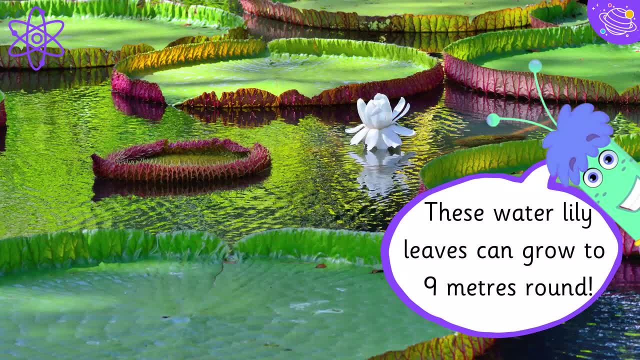 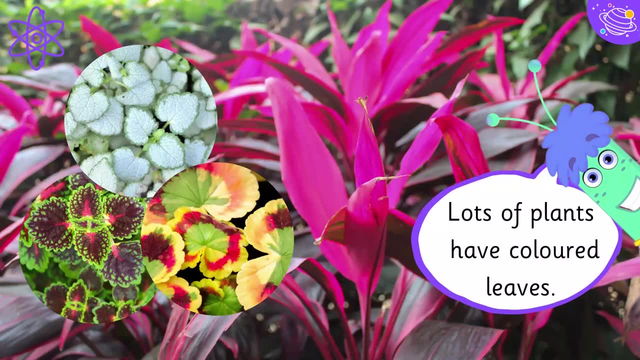 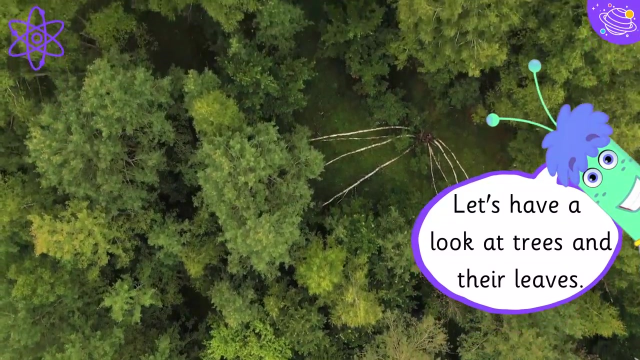 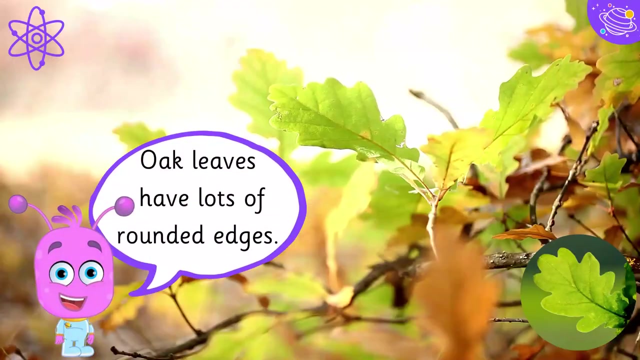 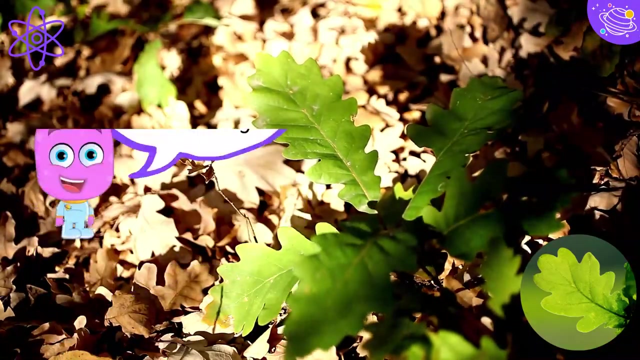 These water lily leaves can grow to 9 metres round. These water lily leaves can grow to 9 metres round. Lots of plants have coloured leaves. Let's have a look at trees and their leaves. Oak leaves have lots of rounded edges. 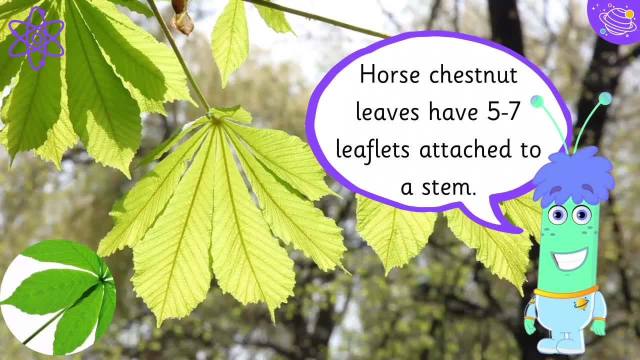 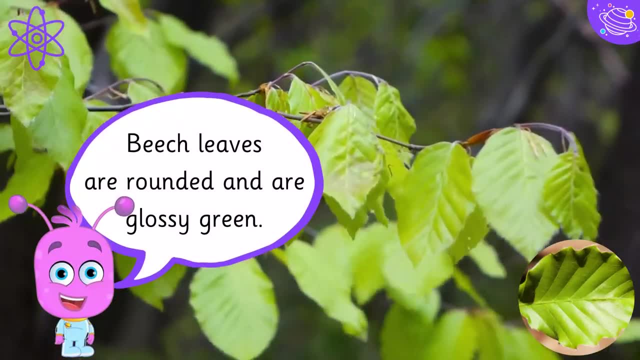 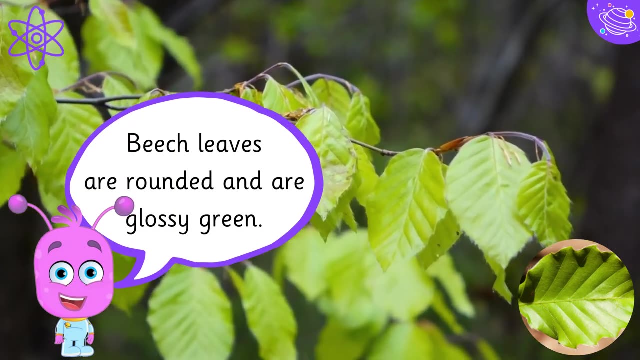 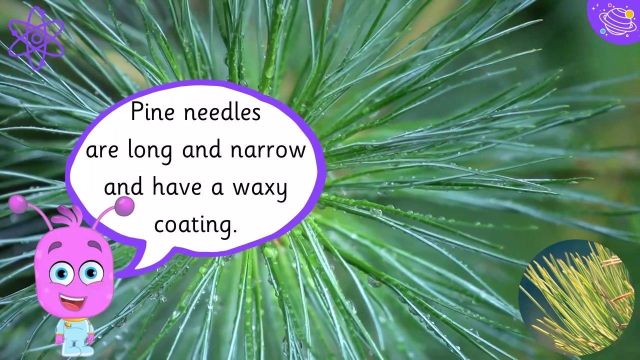 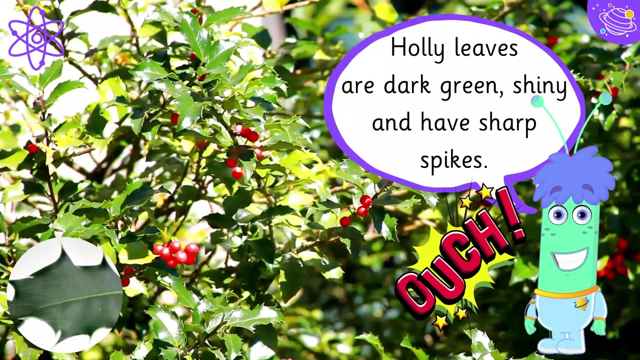 Horse chestnut leaves have 5 to 7 leaflets attached to a stem. Horse chestnut leaves have 5 to 7 leaflets attached to a stem. Beach leaves are rounded and are glossy. green. Pine needles are long and narrow and have a waxy coating. Holly leaves are dark, green, shiny and have 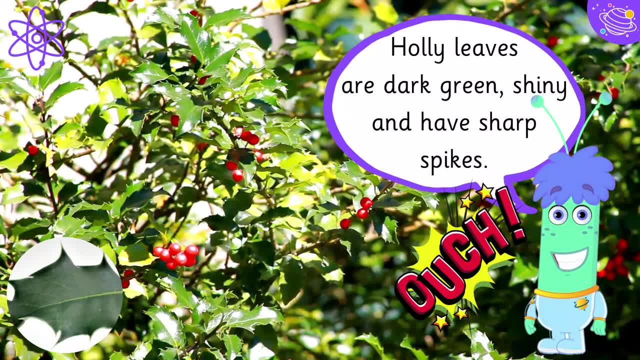 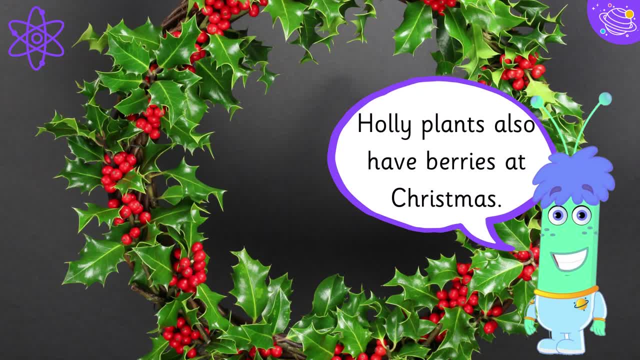 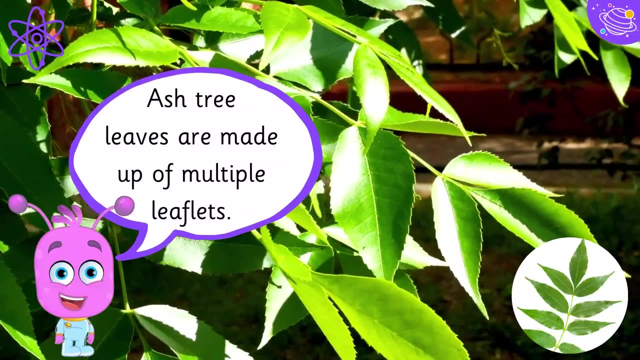 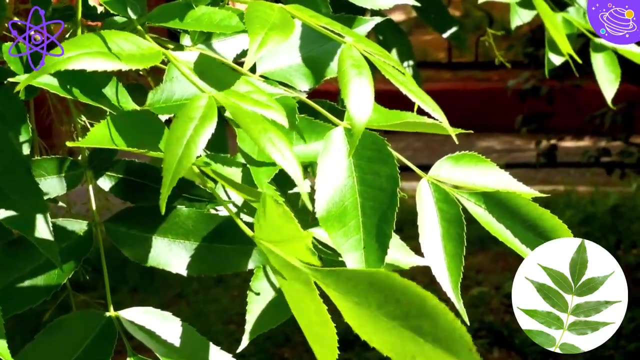 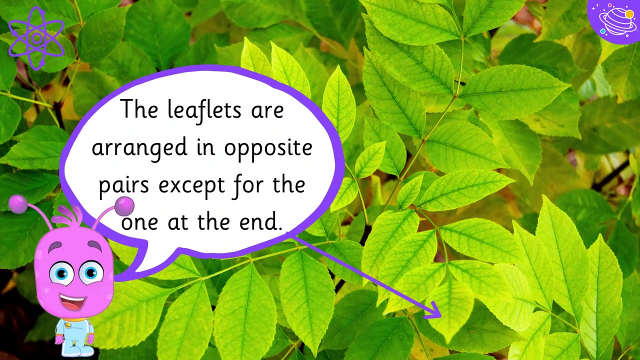 sharp spikes. Ouch Holly plants also have berries at Christmas. Ash tree leaves are made up of multiple leaflets. The leaflets are arranged in opposite pairs, except for the leaves. The leaflets are arranged in opposite pairs, except for the leaves, for the one at the end. 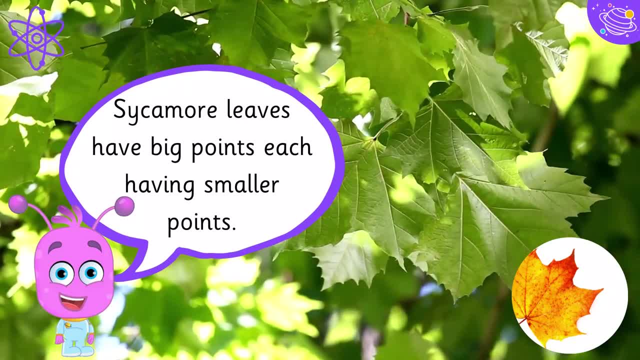 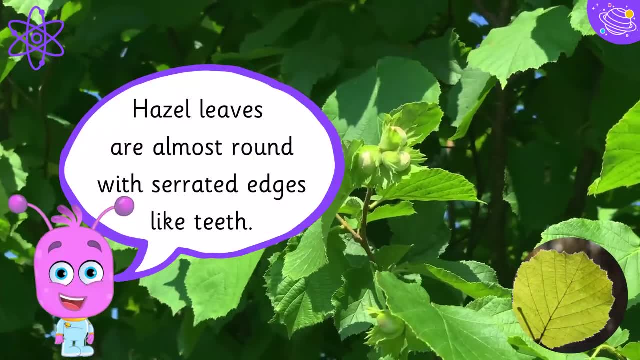 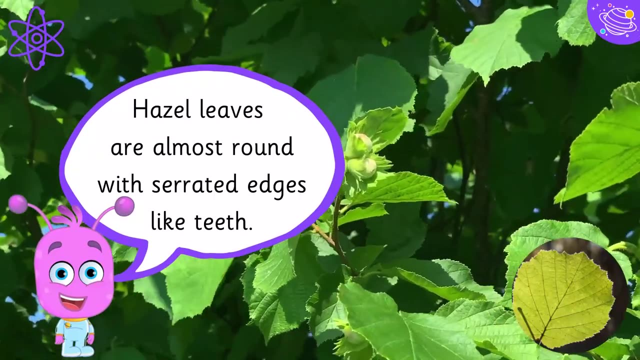 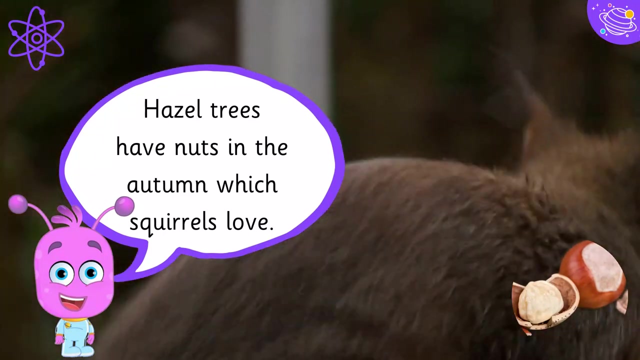 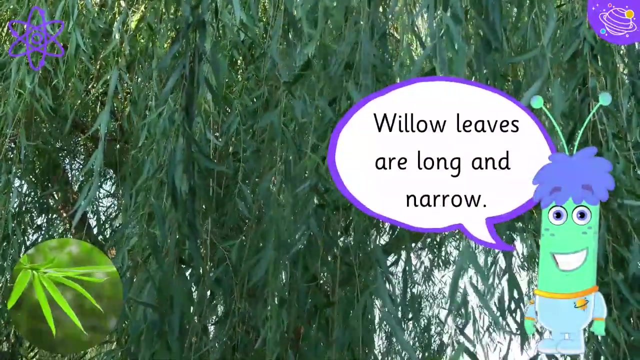 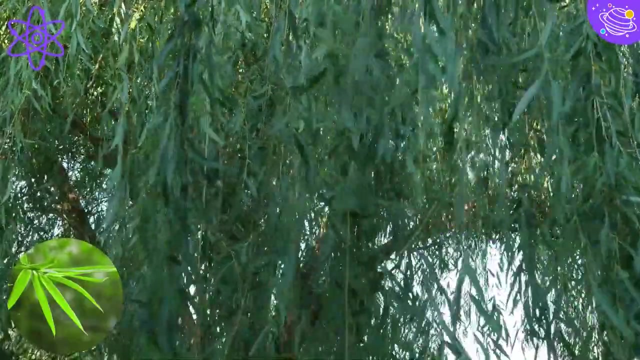 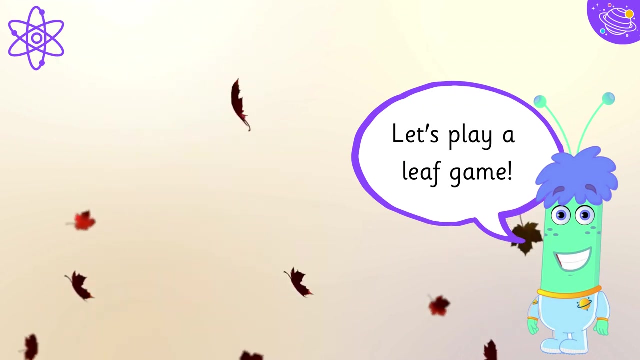 Sycamore leaves have big points, each having smaller points. Hazel leaves are almost round, with serrated edges like teeth. Hazel trees have nuts in the Autumn which squirrels like Willow. leaves are long and narrow. Let's play a leaf game. Well done, Goodbye.